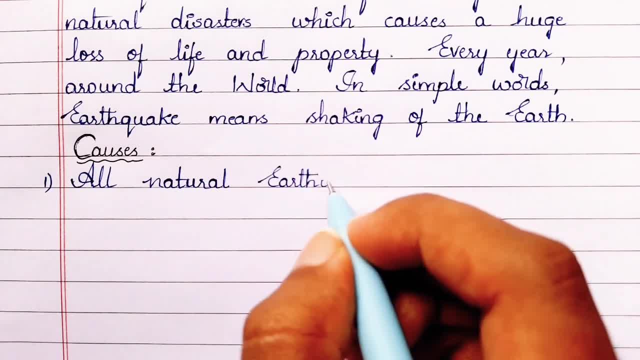 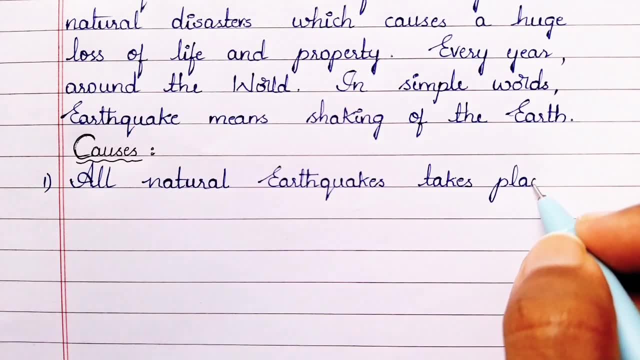 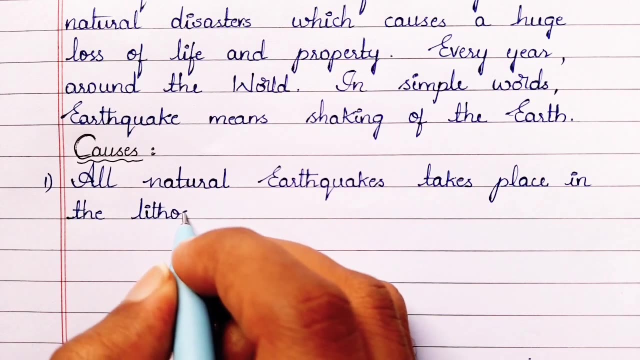 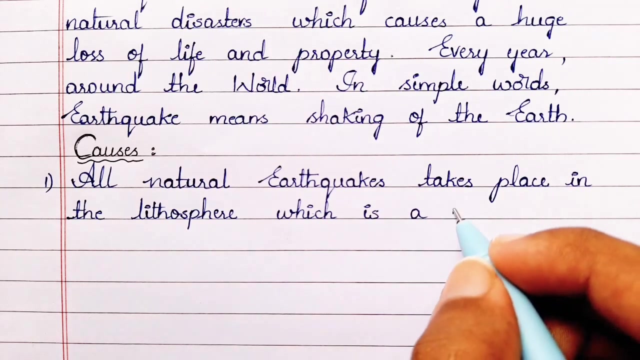 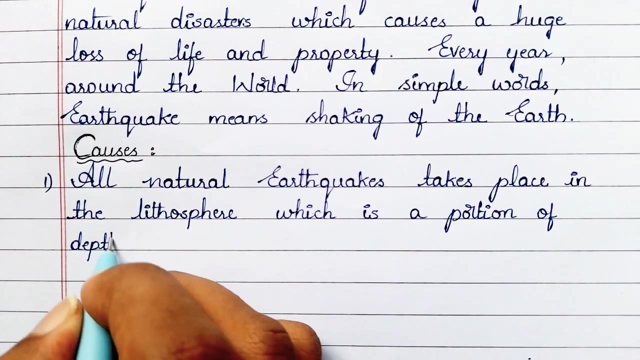 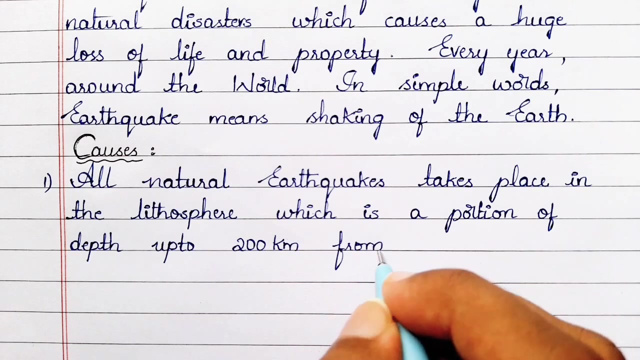 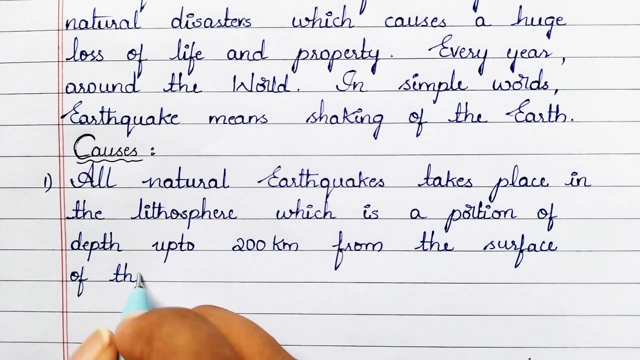 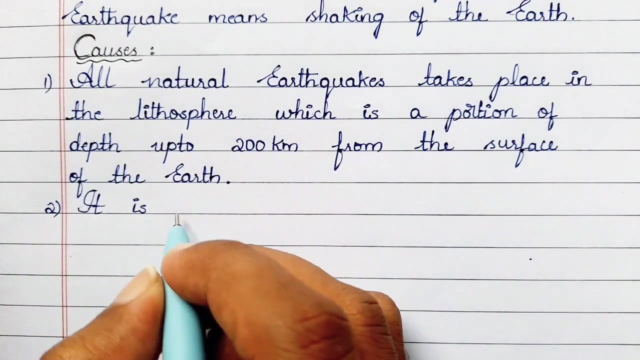 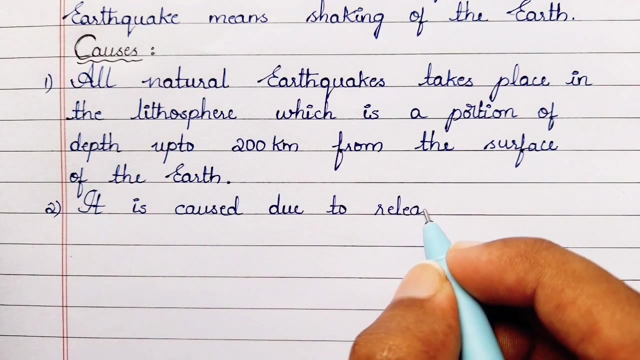 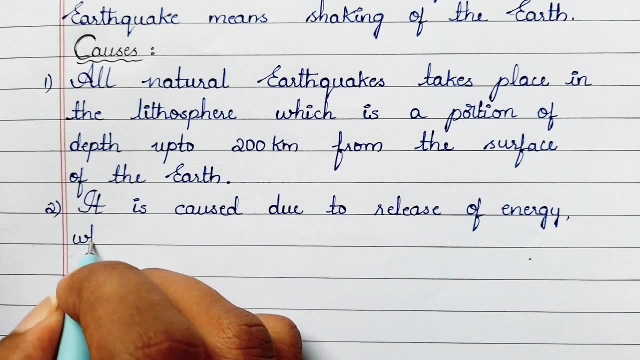 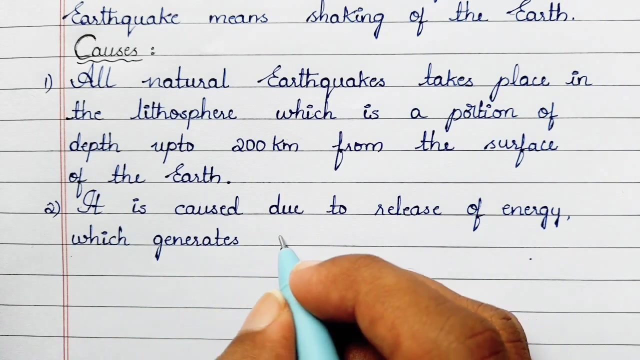 transform. 3. Elevator, when you can see there're constantly aberrations around the earth. 4. All natural earthquakes take place in the lithosphere, which is a portion of depth up to 200 km from the surface of the earth. 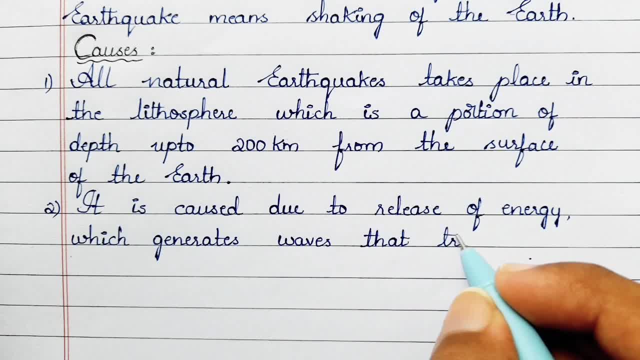 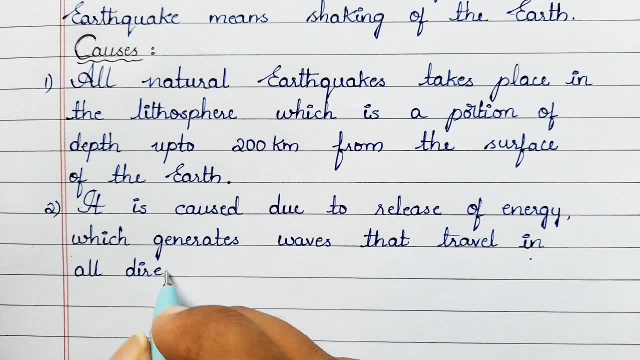 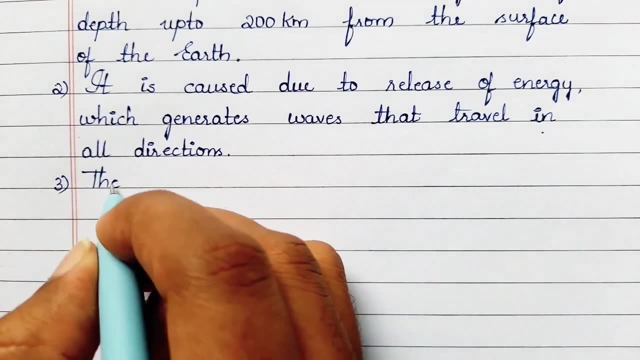 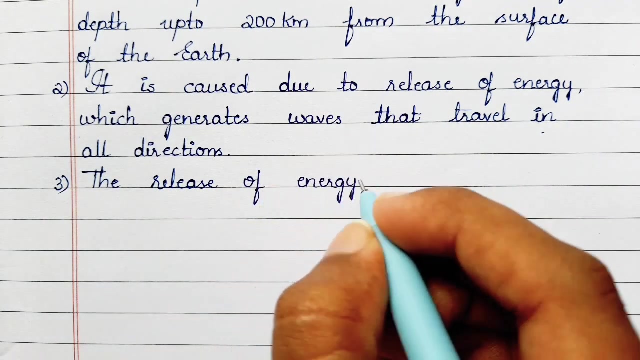 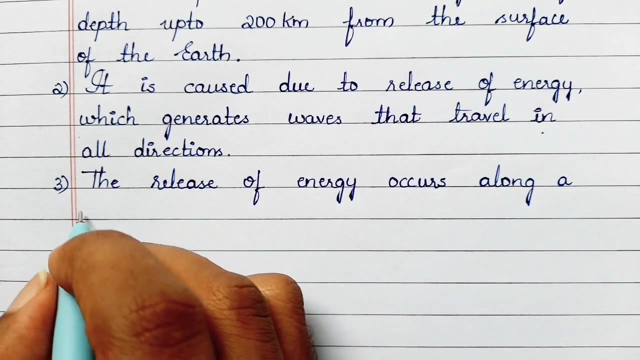 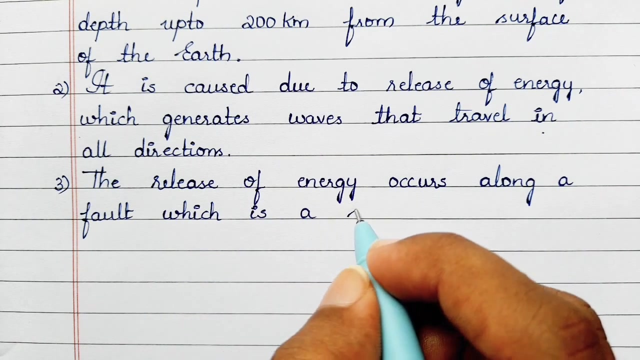 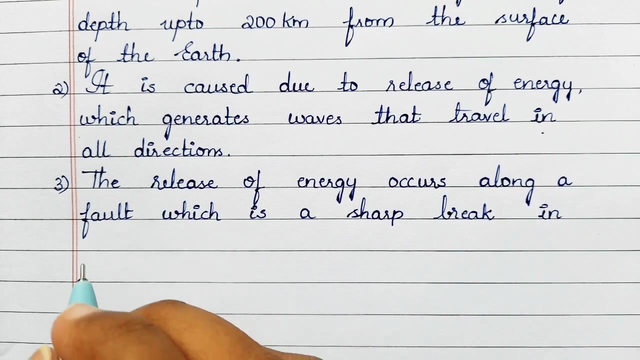 This causes a due to release of energy, which generates waves that travel in all directions, And these waves are said to be seismic waves and mature of two types: P waves and S waves. The release of energy occurs along the fold, which is a sharp break in crustal rocks. 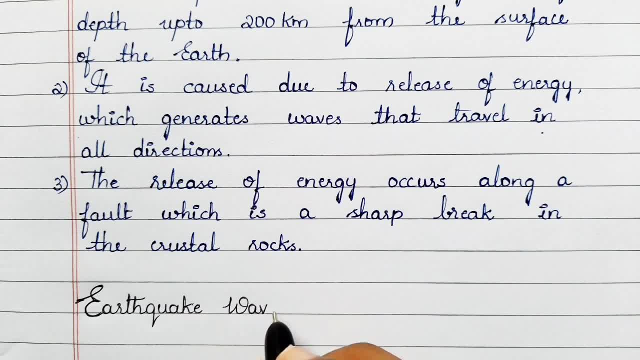 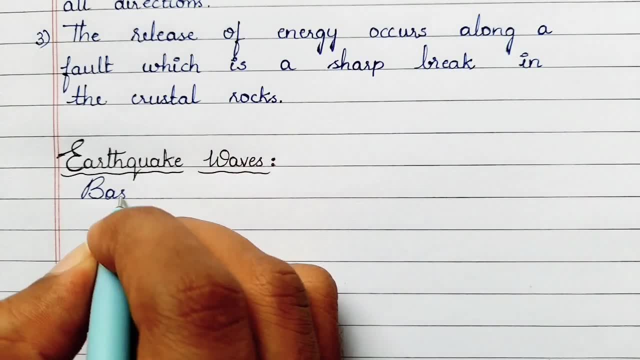 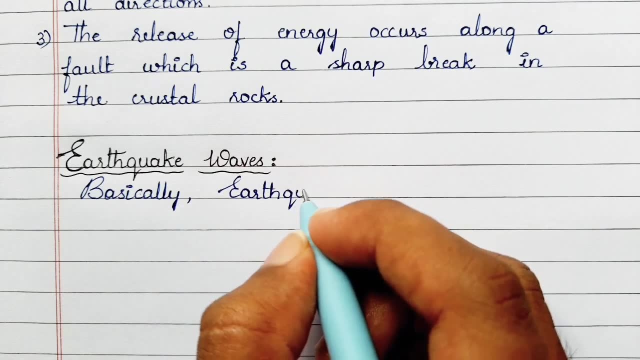 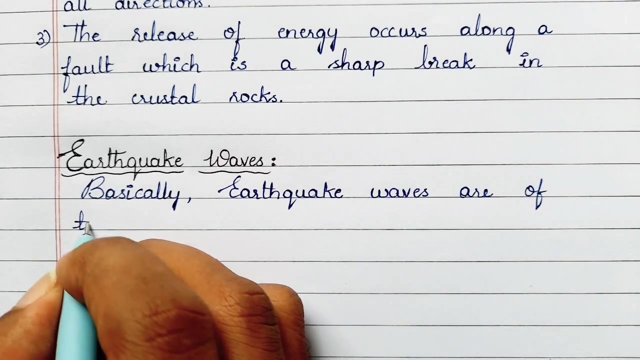 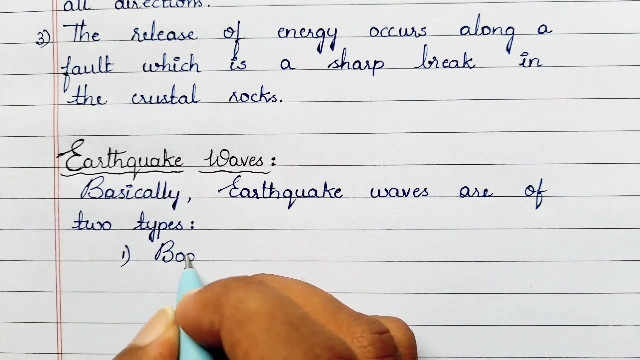 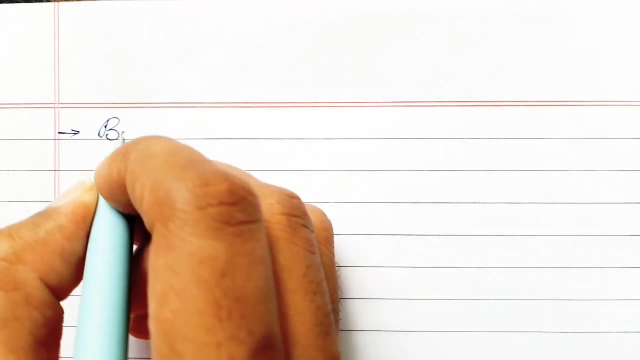 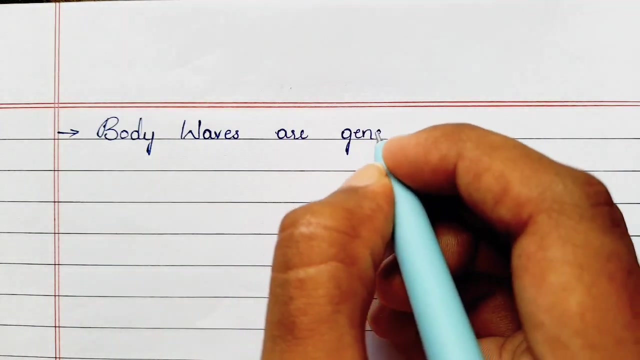 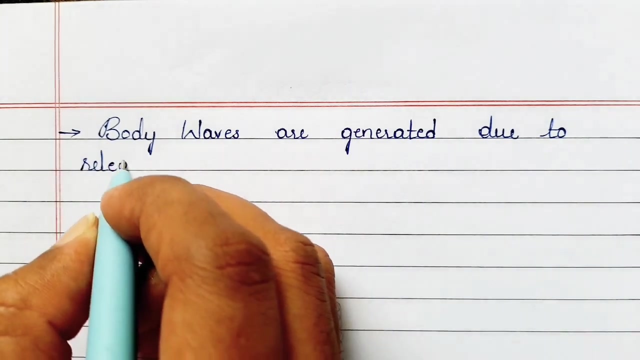 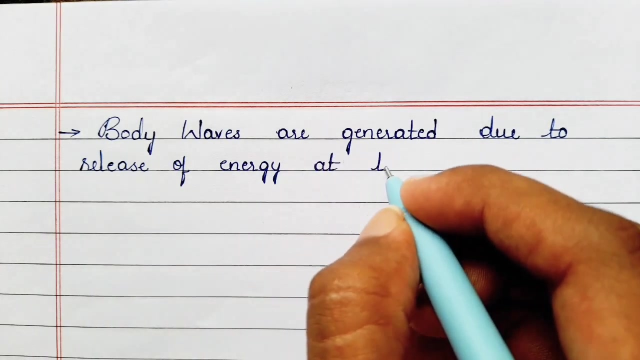 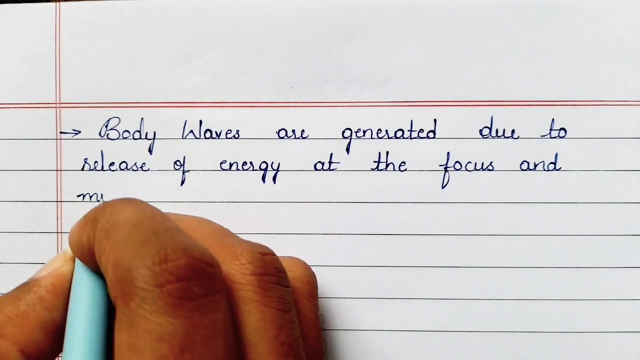 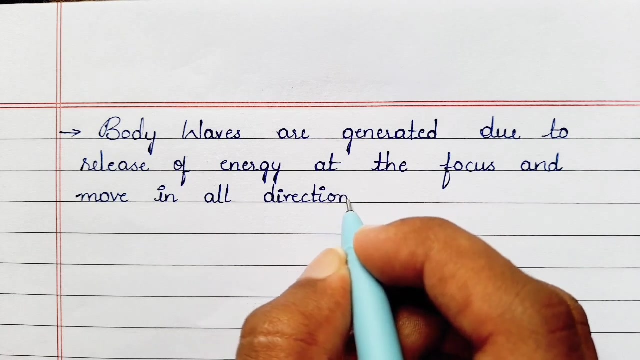 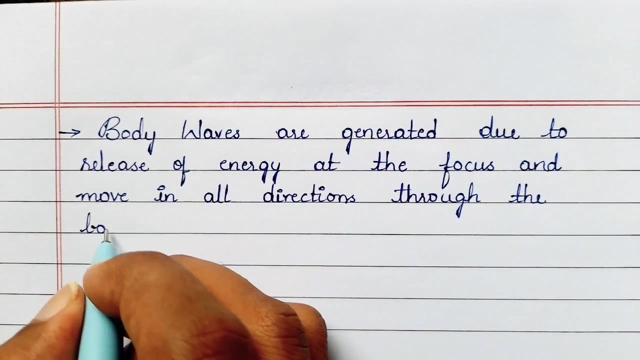 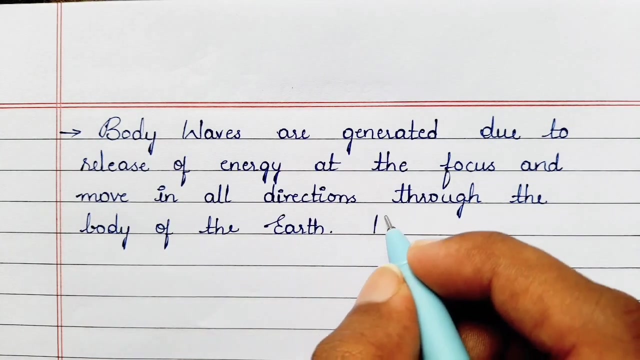 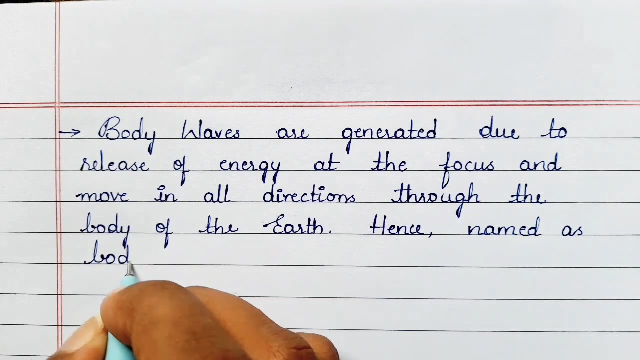 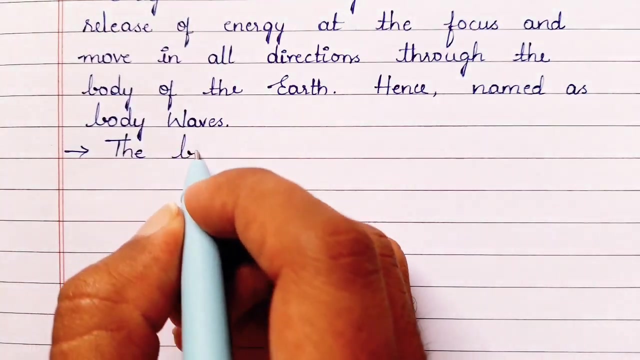 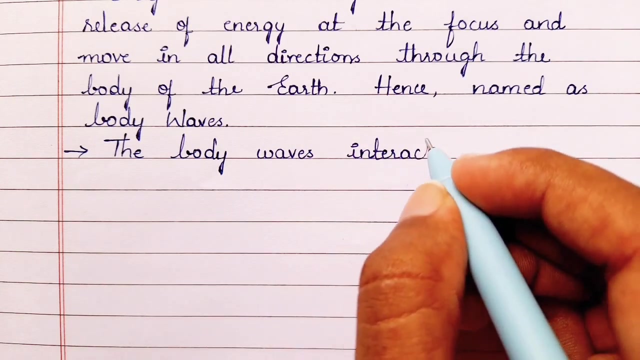 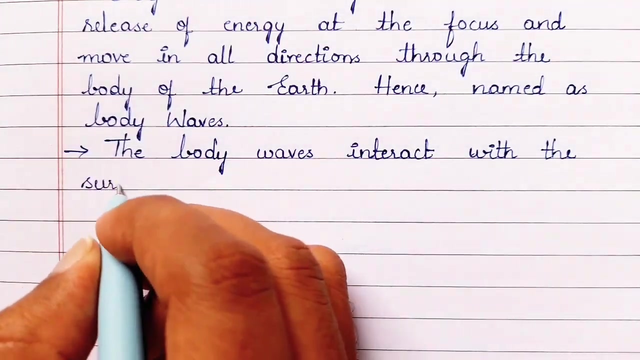 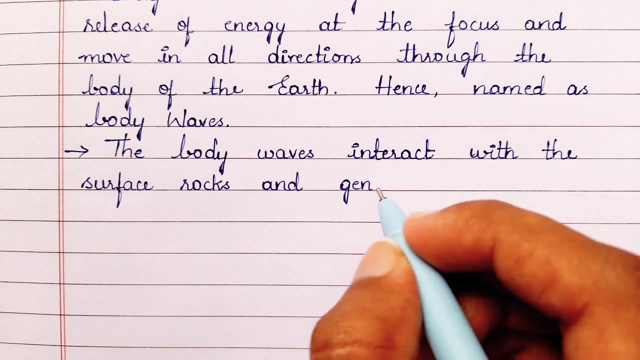 to At Quake Waves. Basically, earthquake waves are of two types: body waves and surface waves. 안녕, Body waves are generated due to the release of energy at the focus and move in all directions through the body of the earth. hence they are named as body waves. 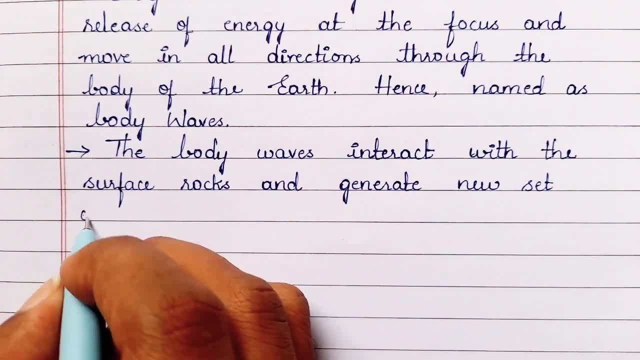 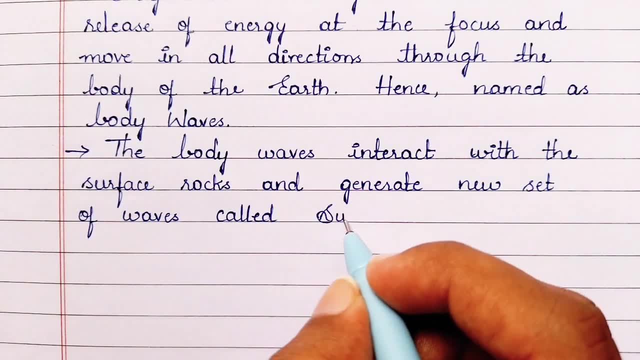 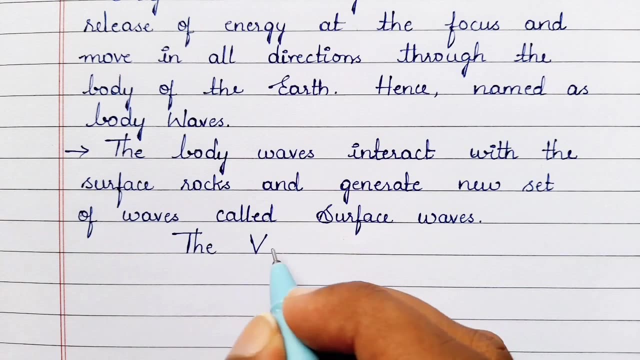 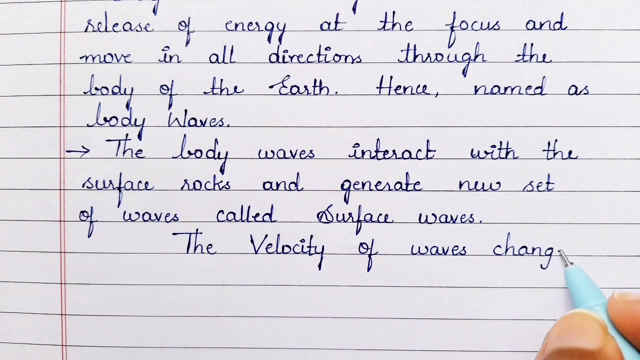 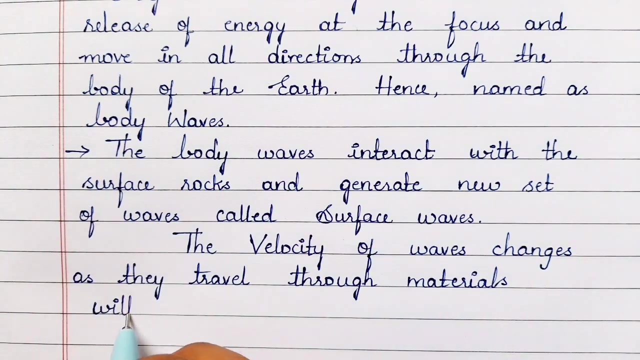 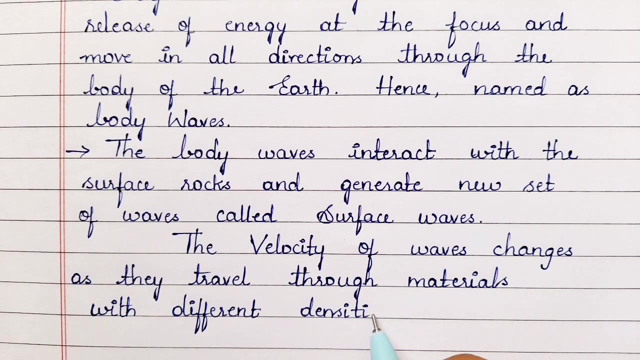 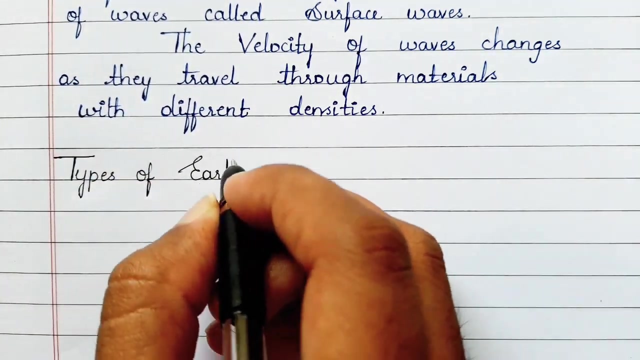 The body, waves interact with the surface rocks and generate new set of waves called surface waves. The velocity of waves changes as they travel through different materials with different densities. And next, coming to the types of uptakes, although it is a natural hazard, the occurrence of uptakes 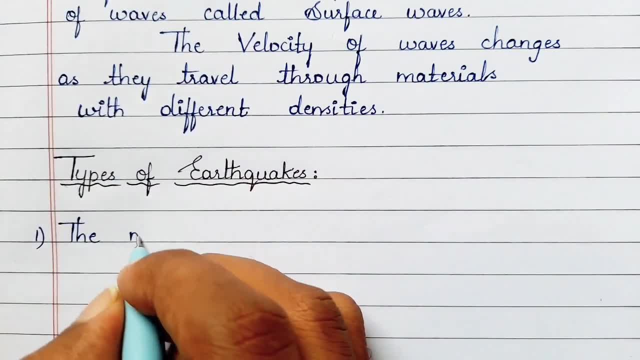 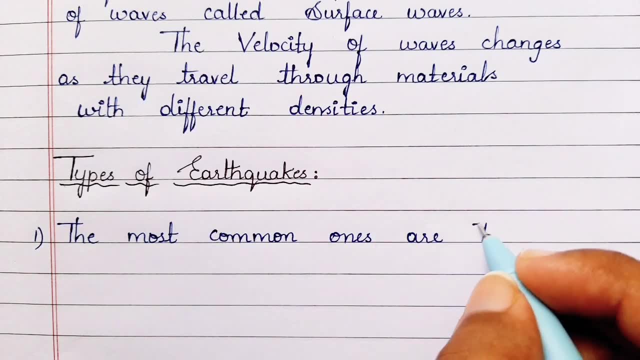 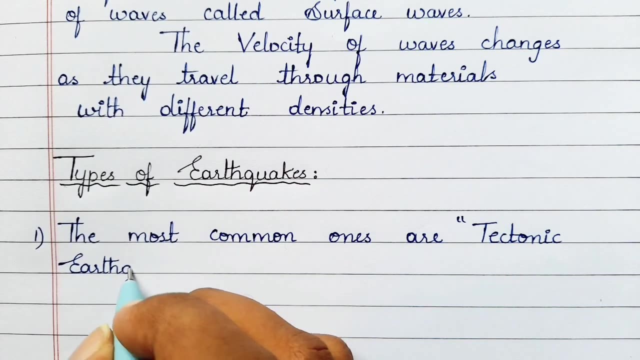 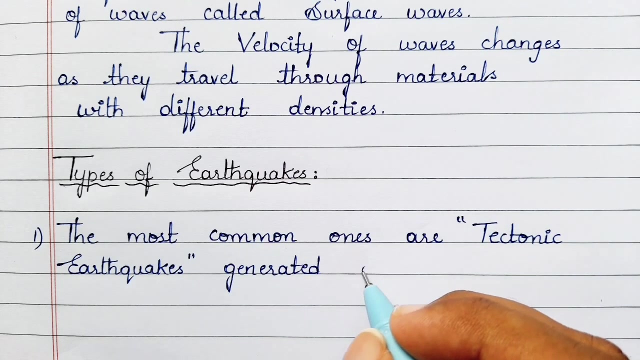 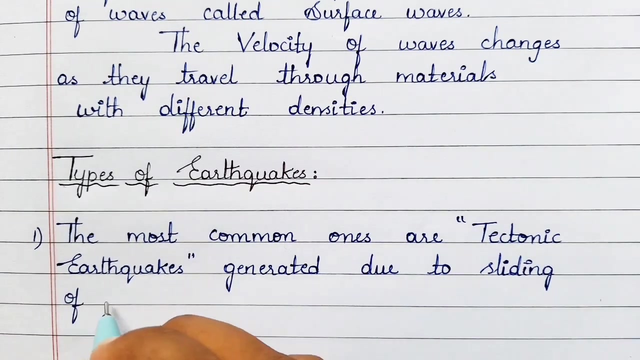 is a natural hazard. The earth is of different types and it is categorized into some types of earthquakes. Regarding theurasic earthquakes, this饅 kosha is the story of 7,000 years ago. The most common earthquakes are tectonic earthquakes. They are generated due to the sliding of rocks along a fault plane. Sometimes the roots of underground mines collapse, causing minor tremors in mining activity areas, and they are called as Collapse Upquakes. Earthquakes that occur in the areas of large reservoirs are referred to as Induced Earthquakes. 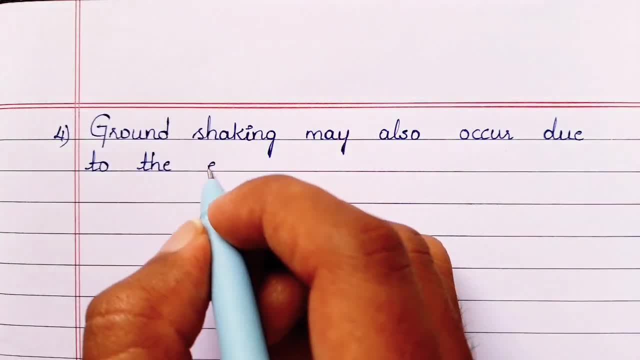 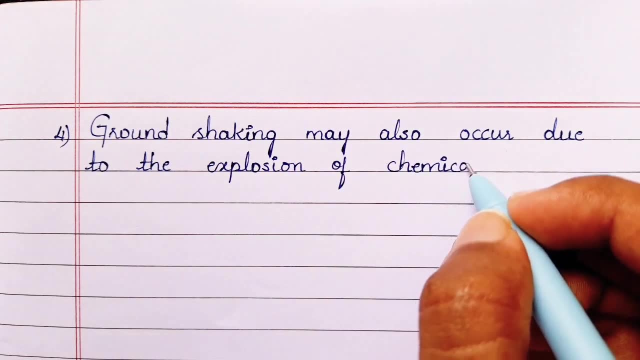 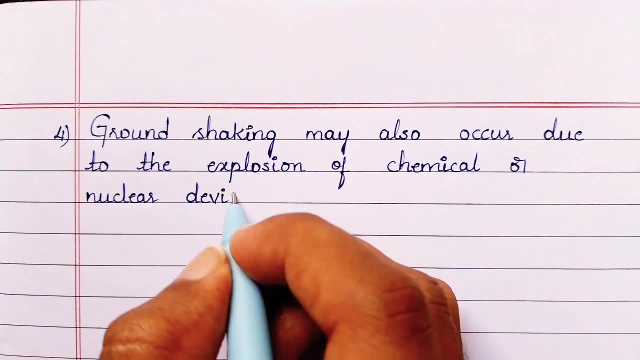 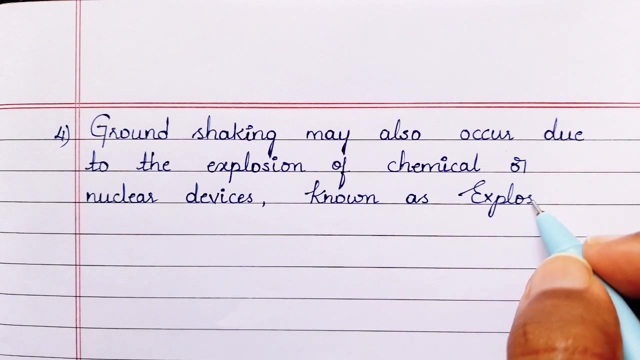 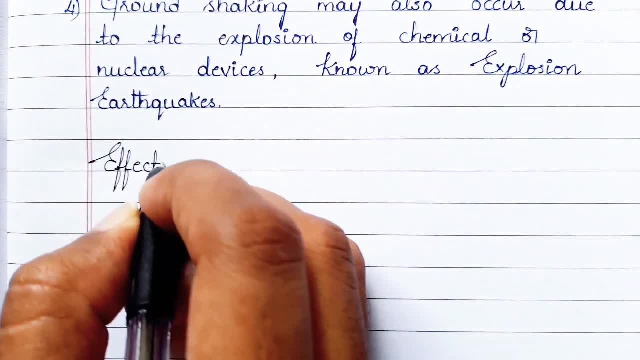 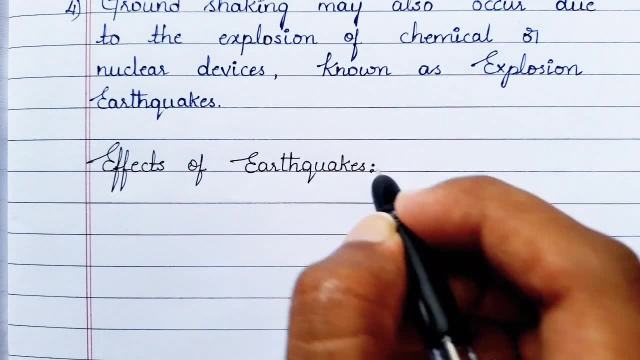 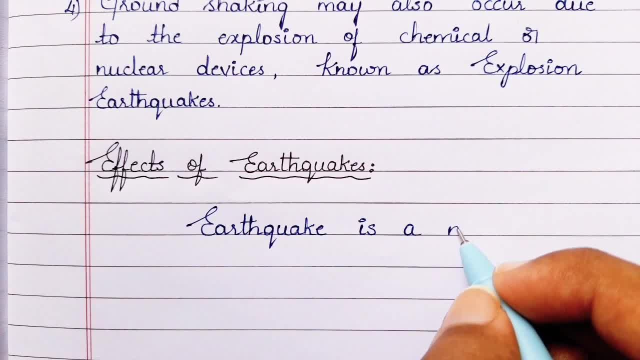 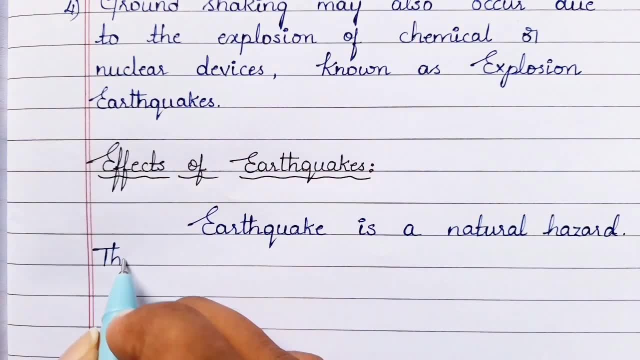 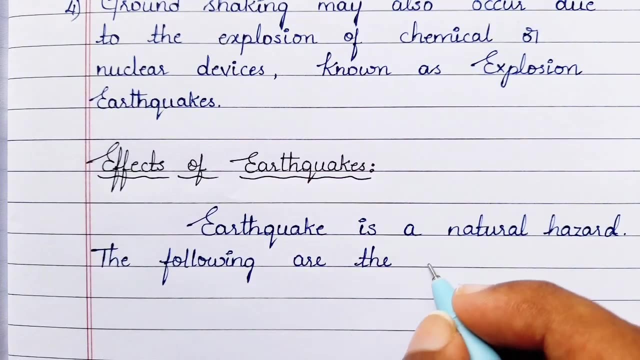 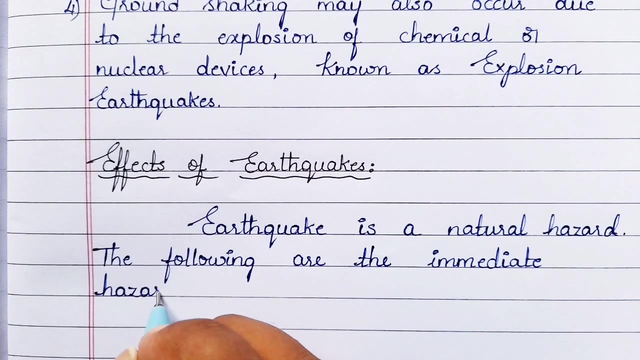 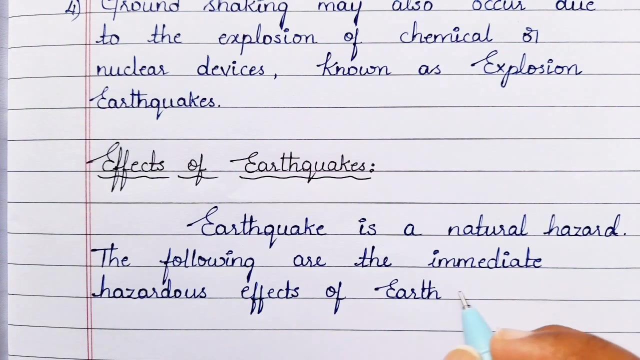 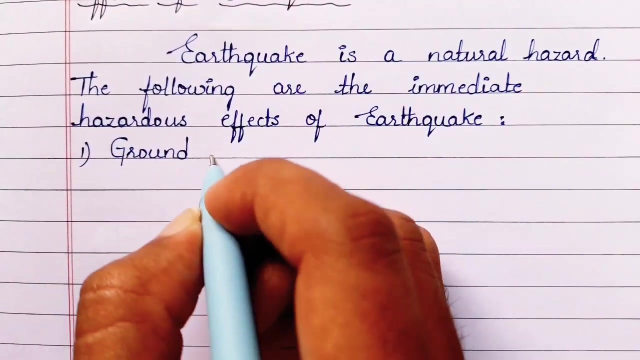 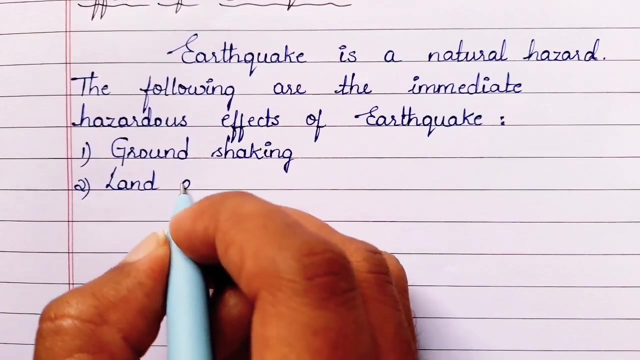 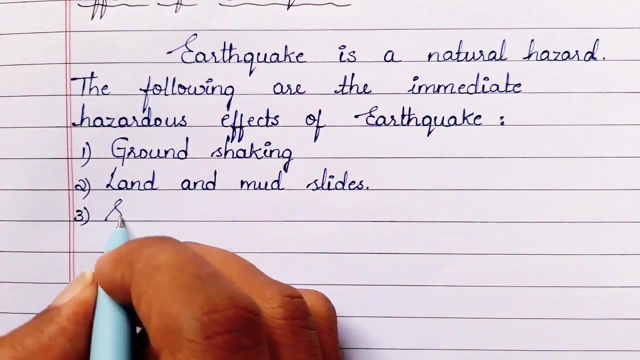 Let's see some of the effects it causes. The first one is Earthquake. earthquake is a natural hazard. the following are the immediate hazardous effects of earthquakes. coming to the first point: ground shaking. it is an immediate effect of earthquakes. land and mud slides, soil liquefaction.